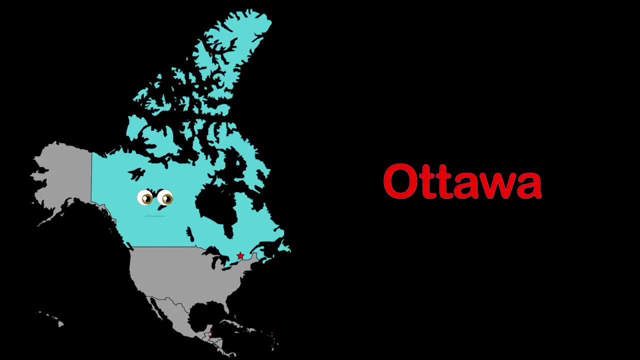 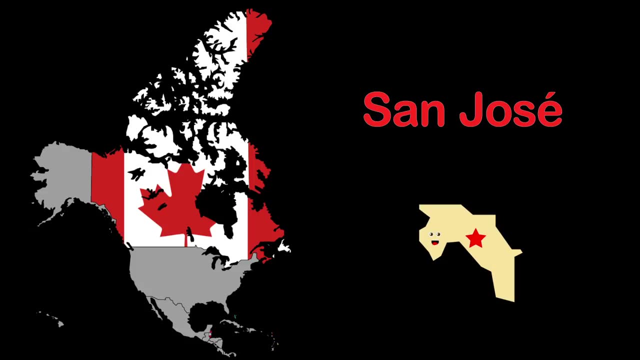 Ottawa is my capital, And this is where it'll be. I'm Costa Rica, Between Panama and Nicaragua. San Jose is my capital. It's where the star you saw. Hi, I am Cuba. I'm off the coast of Florida. I have a capital as well. It's name is Havana. 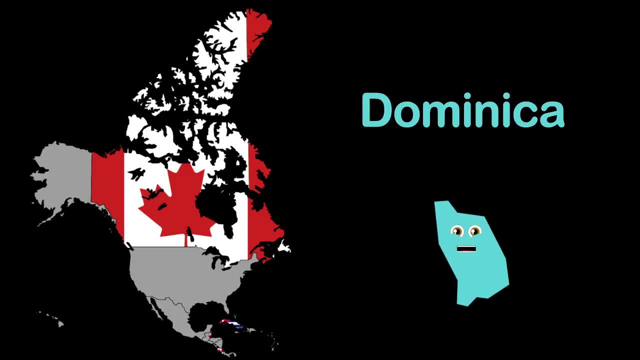 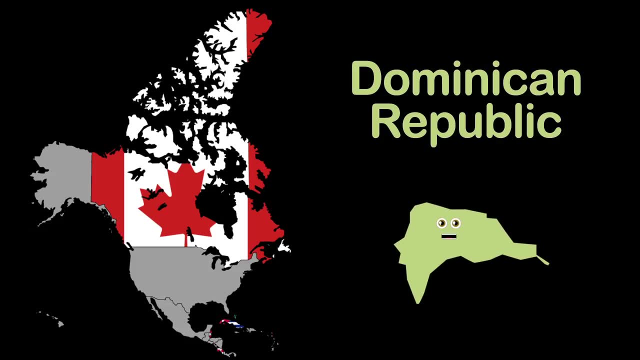 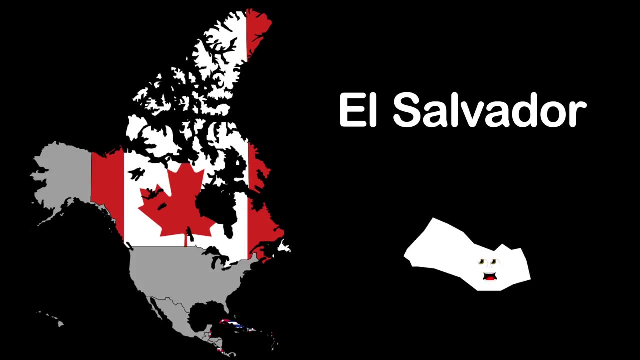 I'm Dominica, A mountainous Caribbean island. Rosso is my capital And this is where it has been. I'm Dominican Republic. I share an island with Haiti, Santa Domingo's, my capital, By the Caribbean Sea. I am El Salvador, The Pacific Ocean. I touch San Salvador's, my capital. 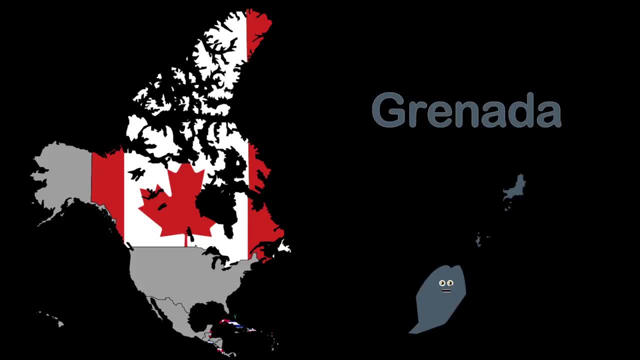 Have you been there that much? Granada, that's me. I'm a Caribbean country. St George is my capital. It's where the star spins that. you see, I'm Guatemala, South of Mexico. Guatemala is the name of my awesome capital. We are the countries of. 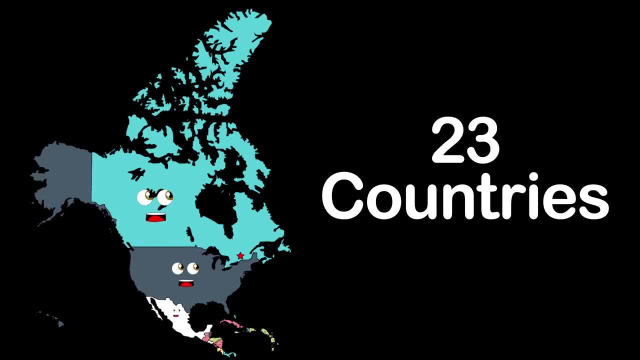 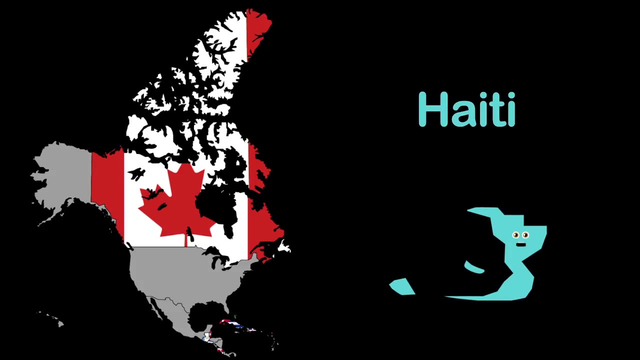 North America- There's 23 presently. We'd love to share with ya. We're the continent of North America Within the Northern Hemisphere. Now sing without a flaw. I'm Haiti. I share an island with the Minico Republic, My capital, Port-au-Prince. Come visit, it's really fantastic. 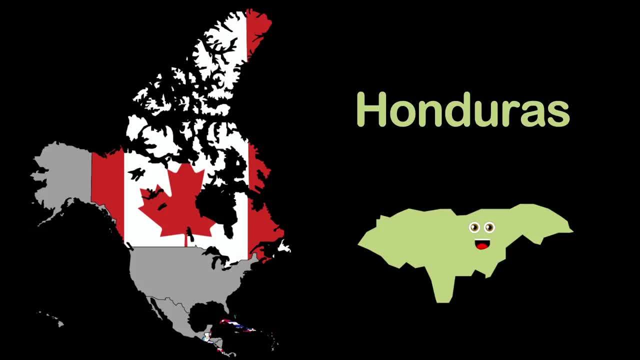 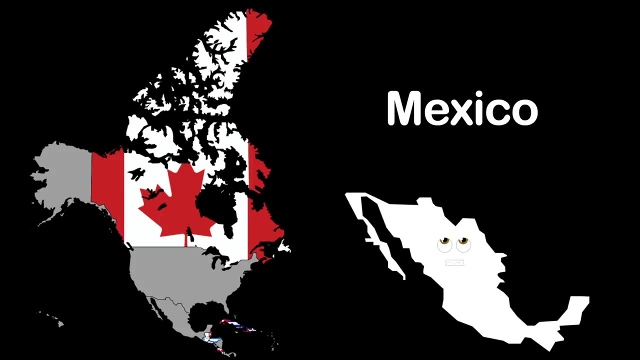 I am Honduras, Right next to El Salvador. Tegucigalpa is my capital. Say it some more, Hey man, I'm Jamaica. A Caribbean island nation To my southeast is my capital. It's name is Kingston. Hola, I am Mexico, South of the USA, you know. 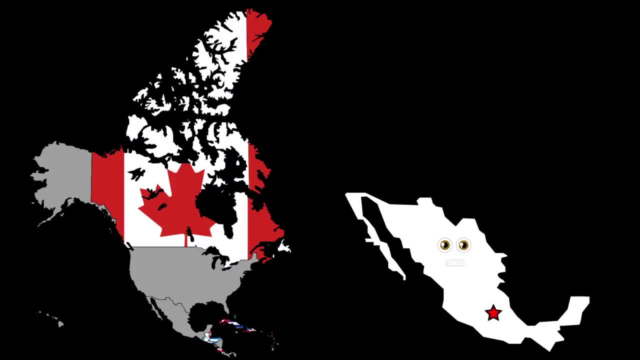 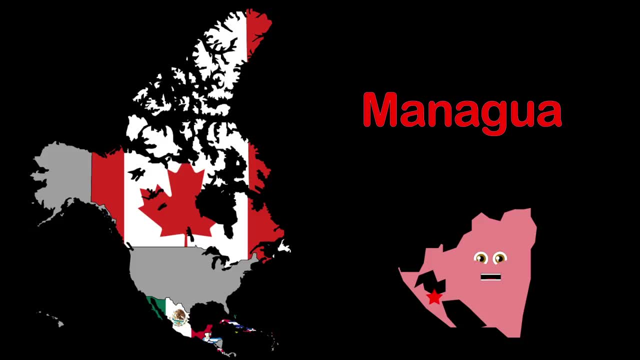 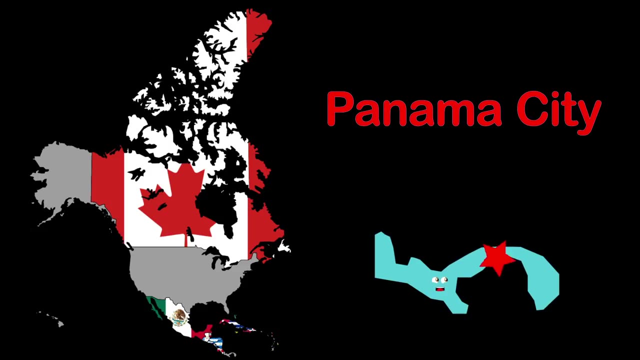 Mexico City is my capital. Maybe someday you will go Nicaragua, here between Costa Rica and Honduras. My capital, Managua, Is a city, and that's a plus. My name's Panama, Home to the Panama Canal. Panama City is the name of My lovely capital. I'm St Kitts and Nevis. 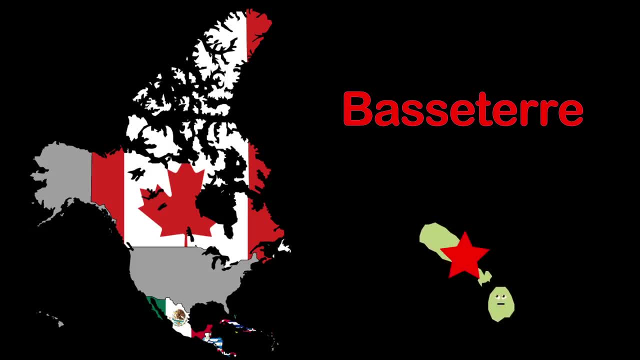 In this Caribbean Sea. Pasadena is my capital. That's a skinny on me. I'm St Lucia, An eastern Caribbean island nation. Cáceres is my capital And my beaches are fun. St Vincent and the Grenadines Is a chain of islands so peaceful.